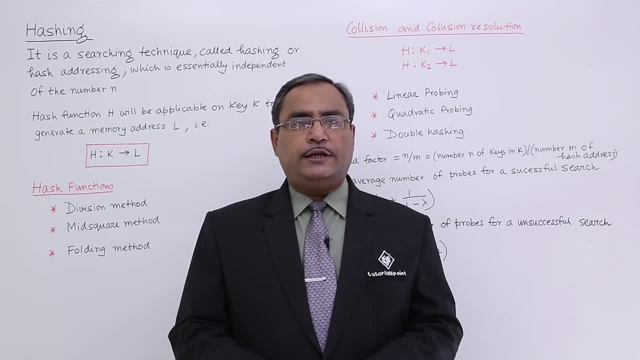 In this session we are discussing a very important searching technique known as hashing. Hashing is nothing but one searching technique, But this particular searching technique is having some uniqueness. We are having a linear search where the searching complexity is of the order of n If you go for the binary search. 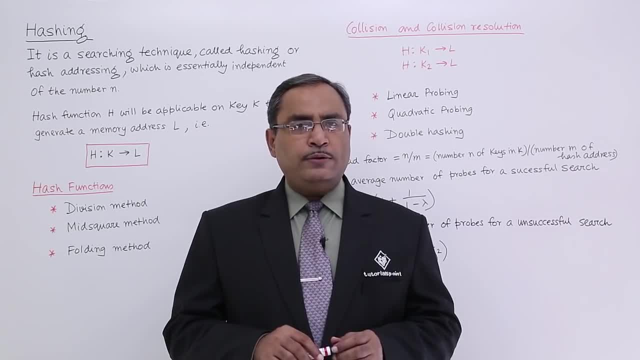 the searching complexity is of the order of log of n to the base 2.. So for those searching algorithms we are getting that the searching algorithm's complexity is depending somehow on the value of n. n means the number of data on which the searching will be carried out. 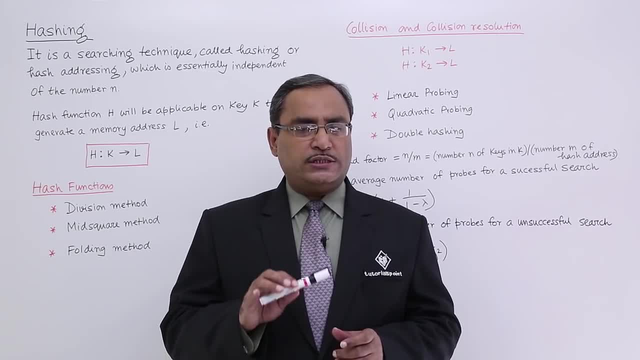 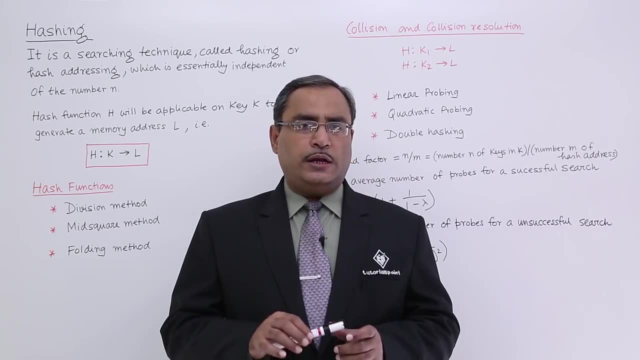 But hashing is a searching technique whose searching complexity is not directly depending on the value of n. So that's why it is one of the most important issues against the searching technique hashing. So here is the text. It is a searching technique. hashing It is a searching technique. hashing It is a searching 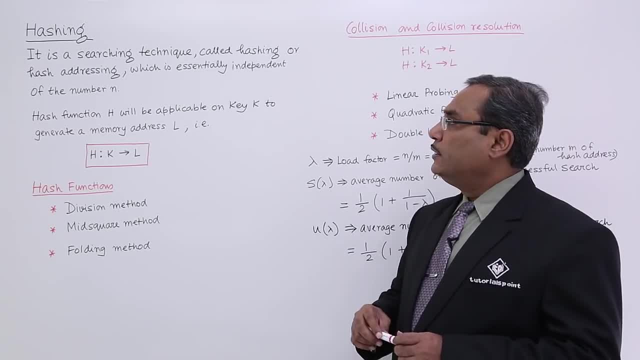 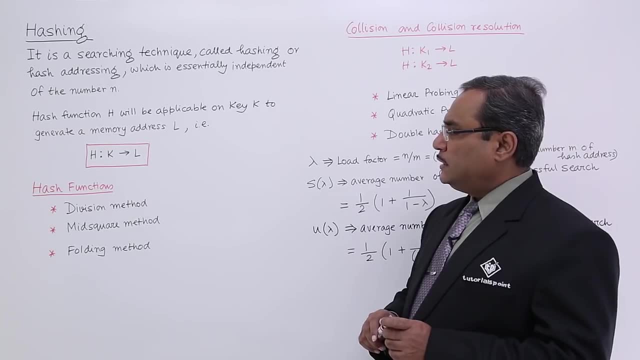 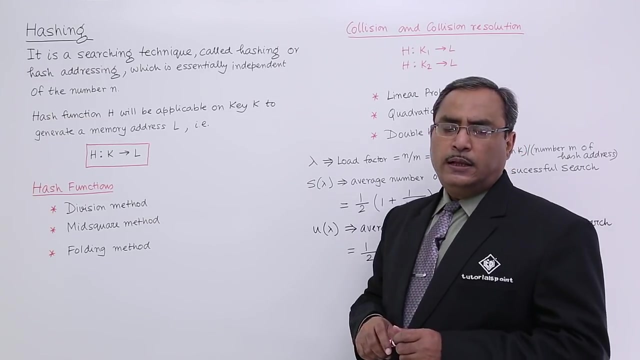 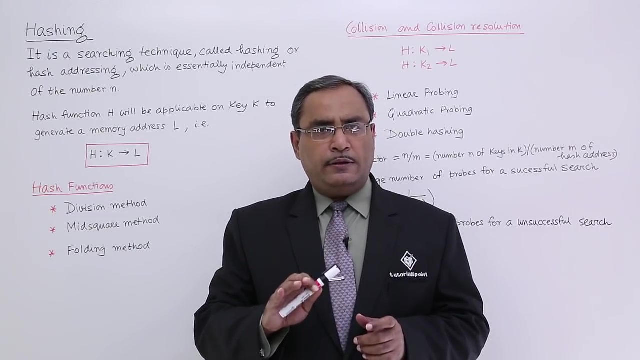 technique called hashing or hash addressing, which is essentially independent of the number of n. So that is very important. Hash function h will be applicable on key k to generate a memory address l. Let us suppose we are having, say, 40 employees And all employees are having four-digit unique. 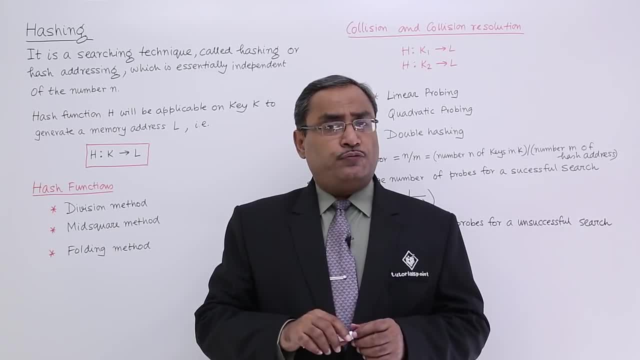 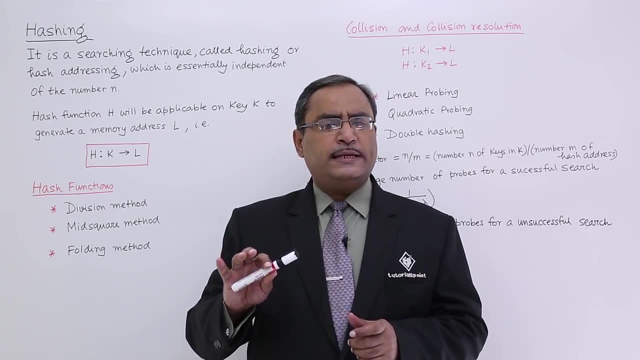 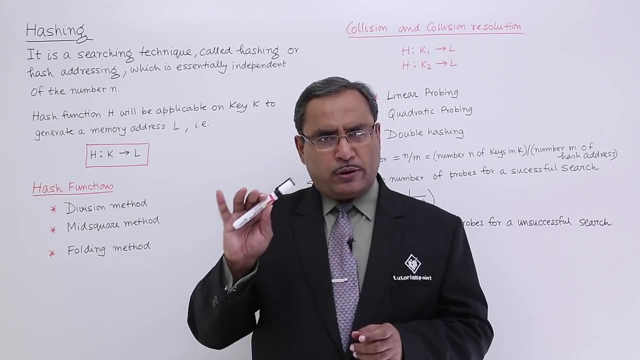 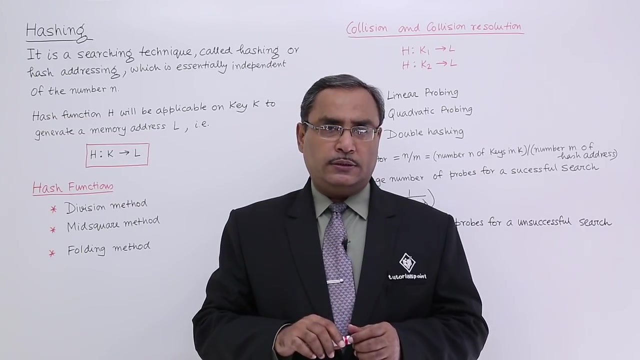 employee code. Okay. So four-digit unique employee code means using four digits We can represent almost 10,000 of different combinations. So using four-digit employee code, we can have almost 10,000 of different combinations, But we are having only 40 employees. So what will happen? 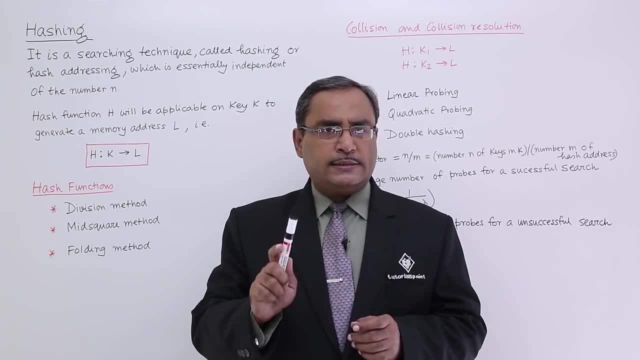 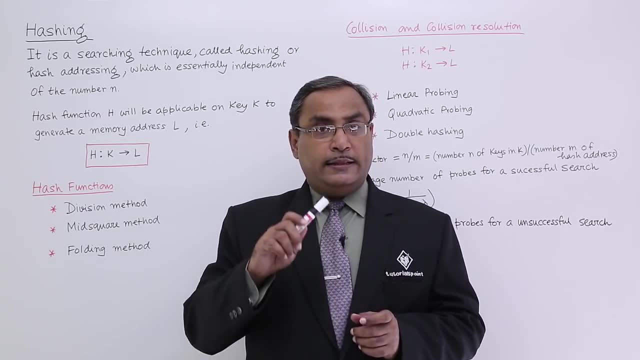 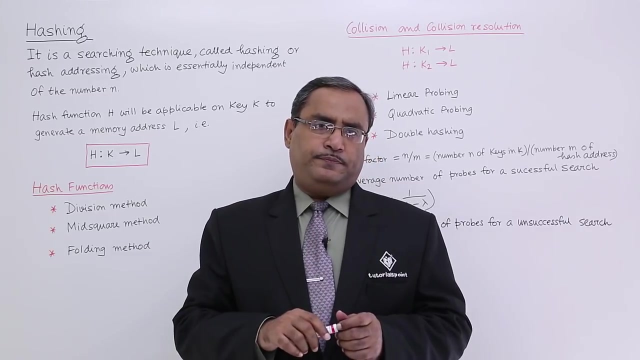 Each and every employee will be having one key value, That is, the employee code. We shall apply some hash function on that employee code k to generate a memory address l. So here is some hash function on that employee code k and then I shall get one l where the respective 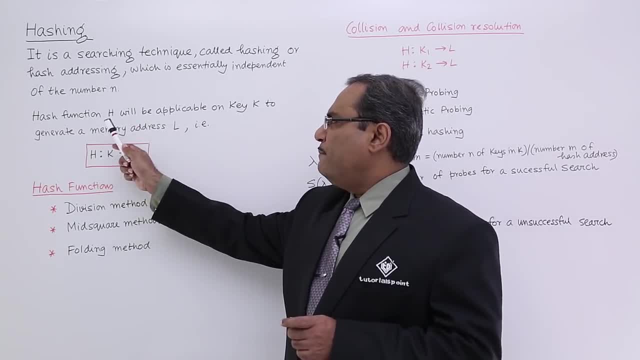 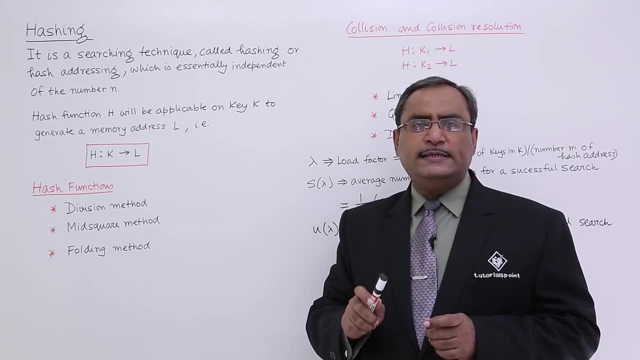 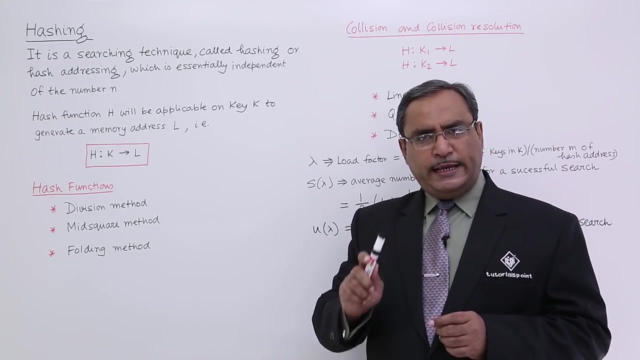 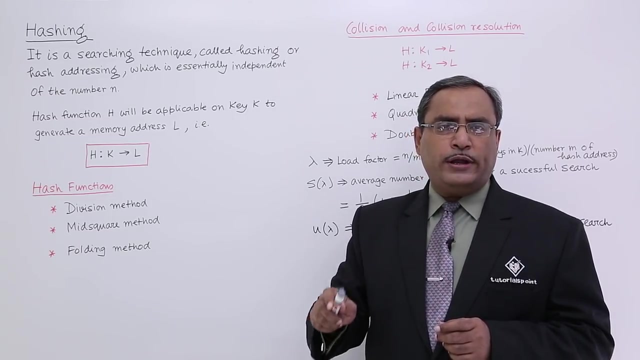 employee details will be kept. Okay, Here is the point. Hashtag function h will be applicable on key, the employee code. why should i call it as a key? because for each and every employee, this employee code is unique. so, using this particular key, we can identify one employee uniquely. so that's why. 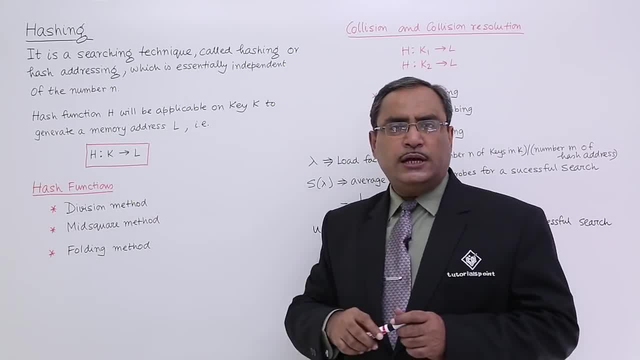 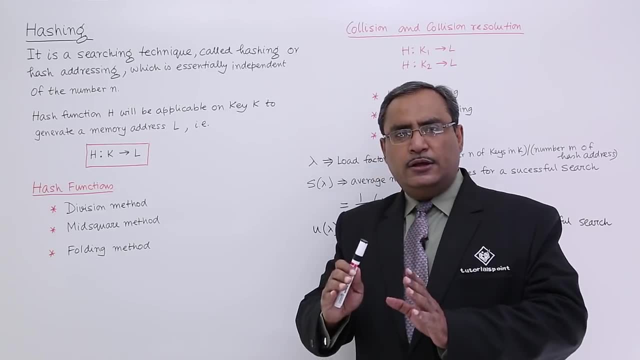 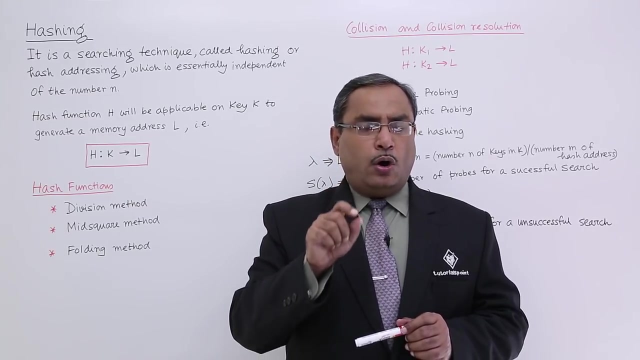 k is a key. and what about? what about this h? h is nothing but one hash function which will apply on, which will be applied on this k, to give me the memory address, l. so what will happen? the four digit employee code will be taken on that particular employee code, one of the hash functions. 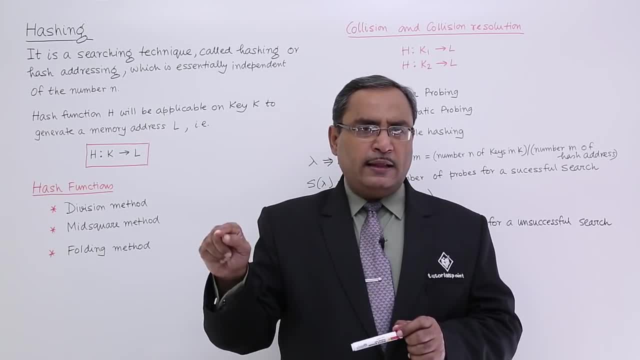 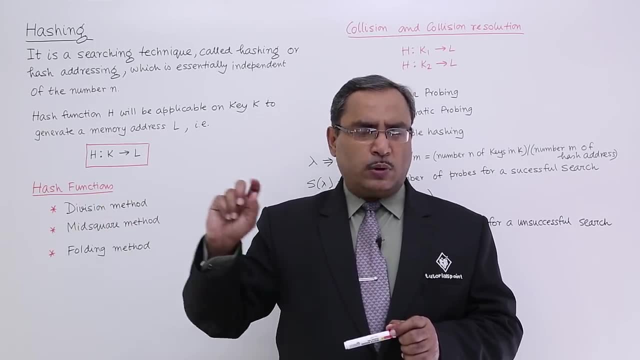 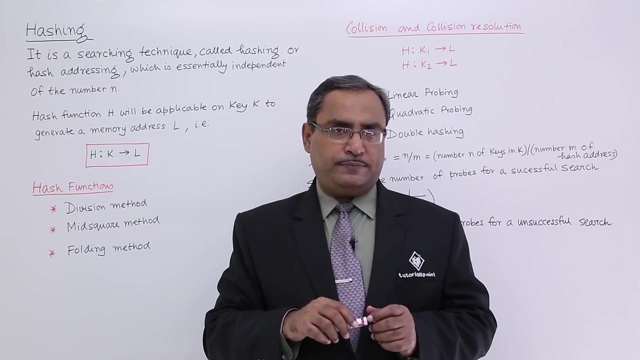 will be applied and then it will give me one l and at the lth location, at the lth location of the memory, we shall be keeping the employee details. whatever the details we require will be keeping there, as usual. so this is known as the hashing. okay, now you might be asking me what are? 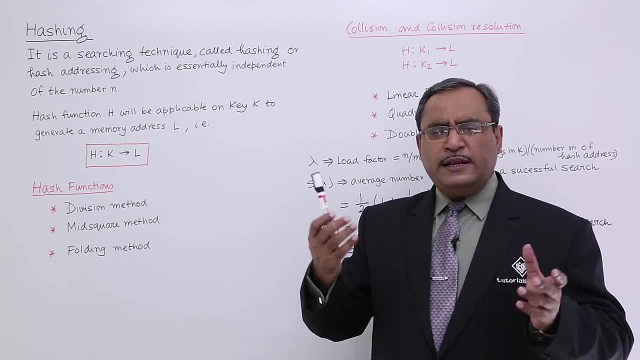 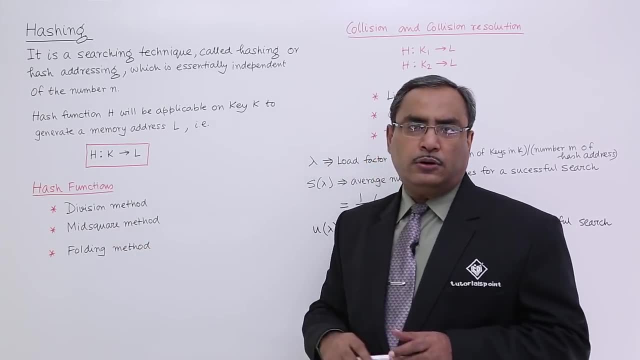 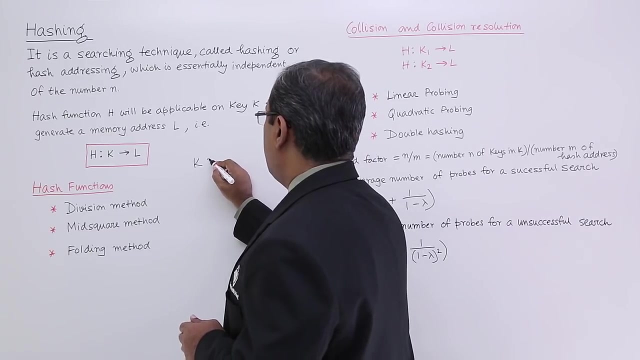 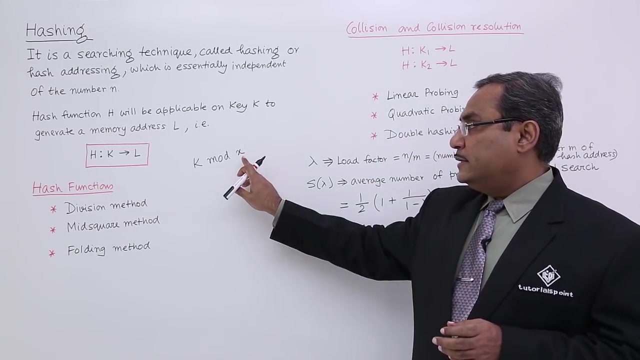 the hashing functions possible. so different hashing functions are possible. some of them are like division method, mid square method or folding method. now, what is a division method? division method is very simple. i can write in this way: say k mod of say x, so x is a value which will be applied here, so k mod x. so that means i shall. 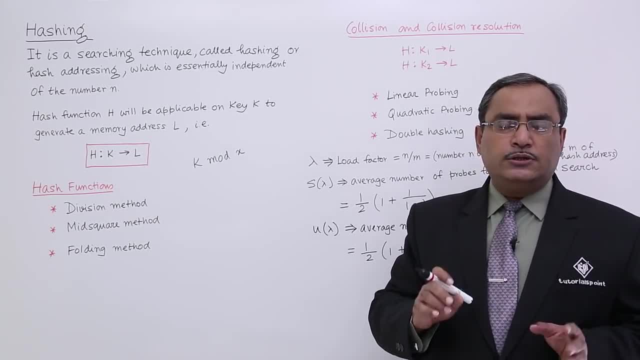 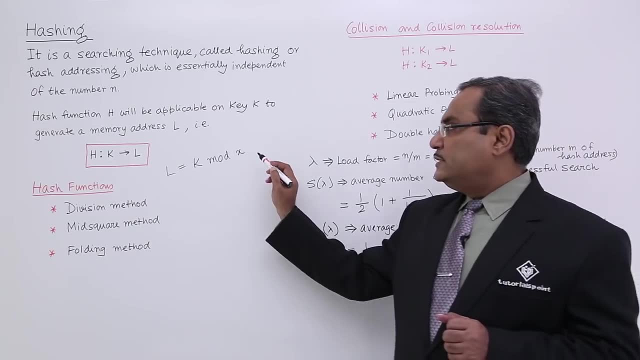 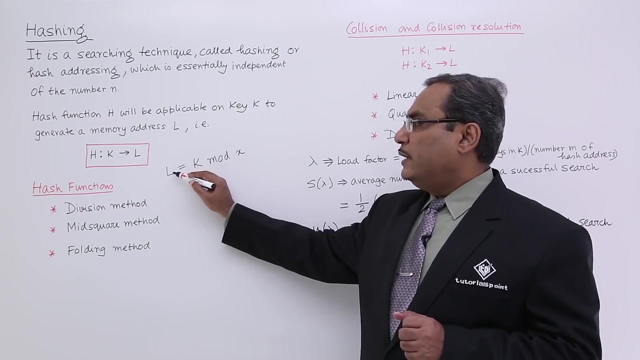 divide k by x, i shall take the remainder. so if i take the remainder, then then at that very location, and that will give me l, that is give me l. so this is my h of k, that is a hashing function on k. so k mod x will give me the value l and at that very location, all the employee details. 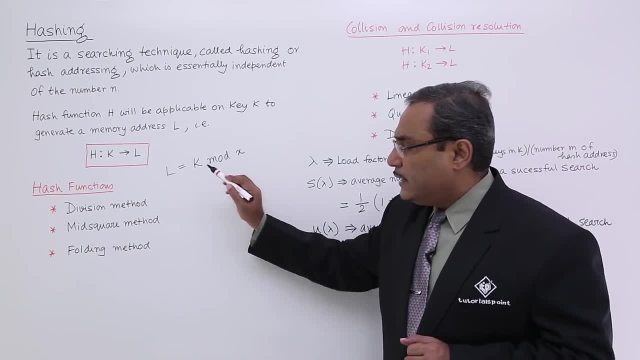 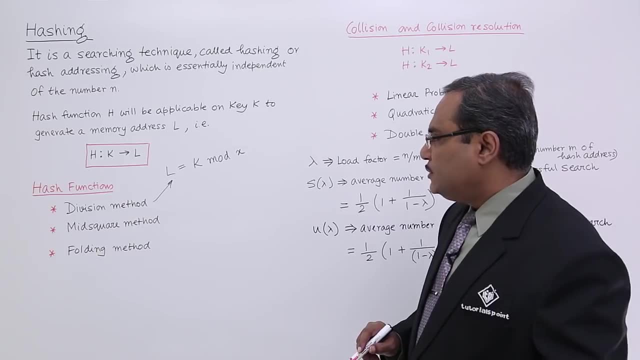 employee details respectively to that particular k value will be kept. so that is my division method. if you go for the mid square method, if you go for the mid square method, it will be something like this. i'm just telling you. let us say that i have a k value, and i have a k value and i have a. 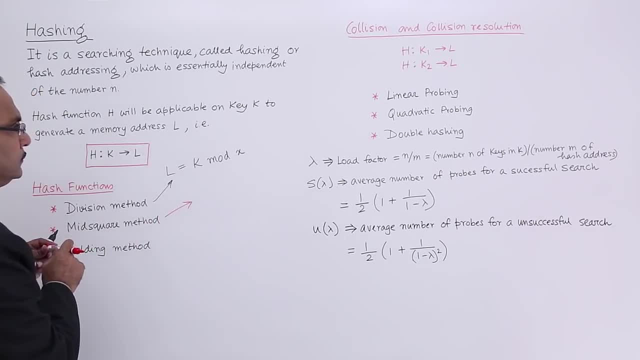 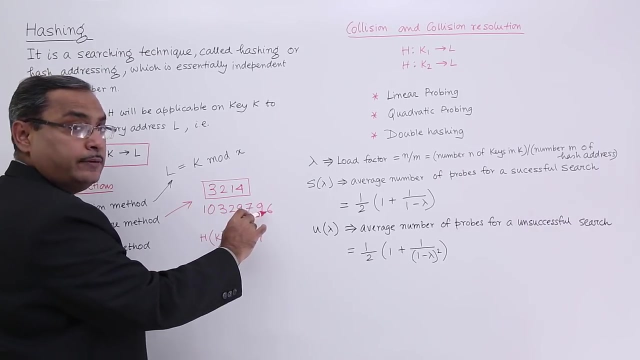 k value. so let us suppose we are having one employee code like 3214. if you go for its square it will be like this: that means in case of mid square method, let us suppose this four digit employee code is 3214. so here the square has been taken, so it is nothing but. 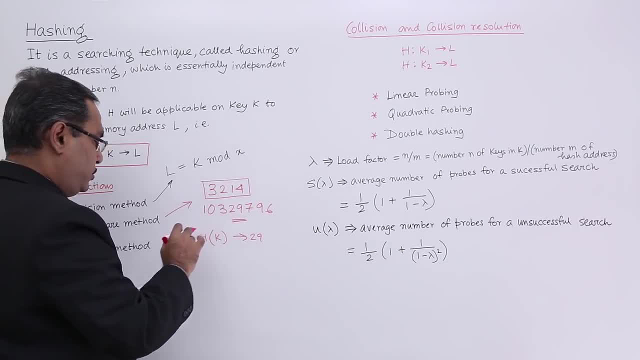 3214 whole square. so that is the value in case of mid square method. i shall discard, say, three digits from the left hand side and three digits from the right hand side. i shall take this 29 and that is my mid square method, that is my. 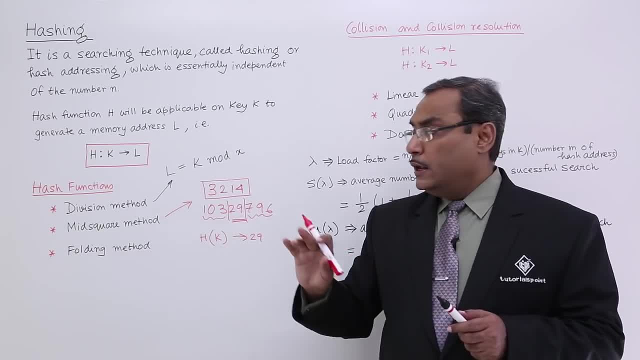 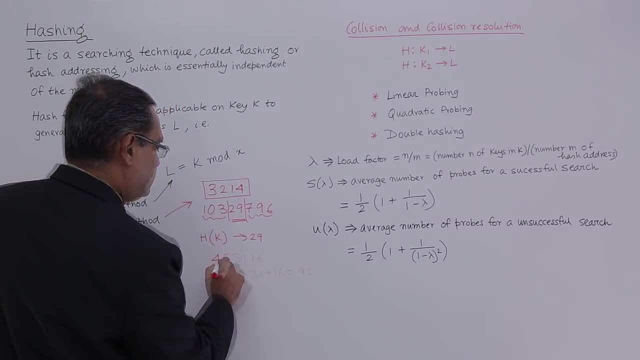 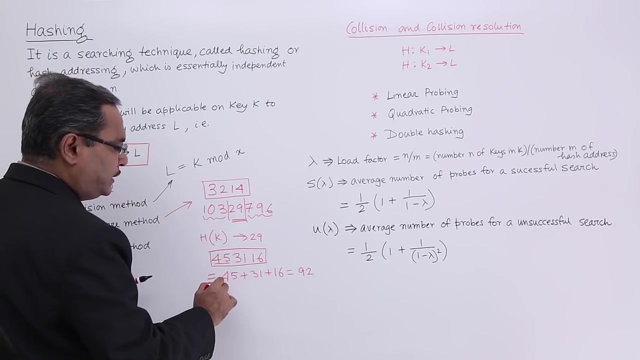 mid square method. so in this way it will be taken. now, in case of folding method, what will happen? let me take one example here. let us suppose the employee code is something like this: now i shall go on adding two digits, two digits and these two digits. i'm getting this particular value and that is my l, if i get one. 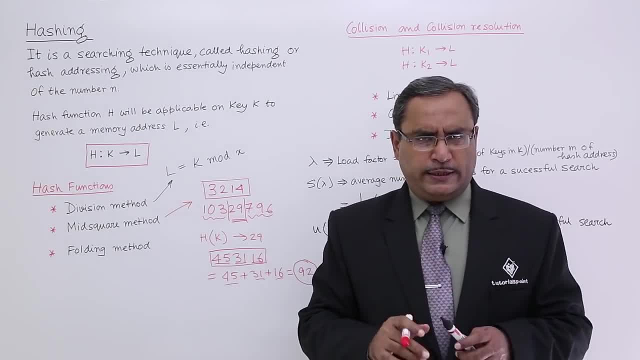 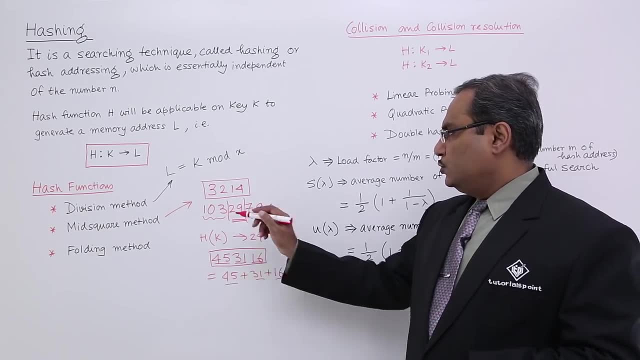 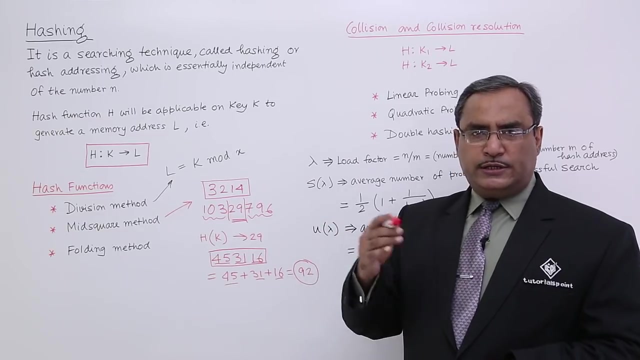 remainder i can also discard. so whatever we are thinking about, this particular hash functions accordingly. i shall be getting the value of l. so 3214. mid square means i'm just doing the square and taking the middle most two digits. so that's why it is called mid square. in case of folding, 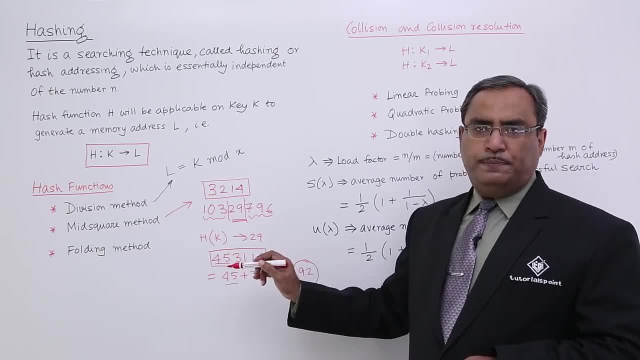 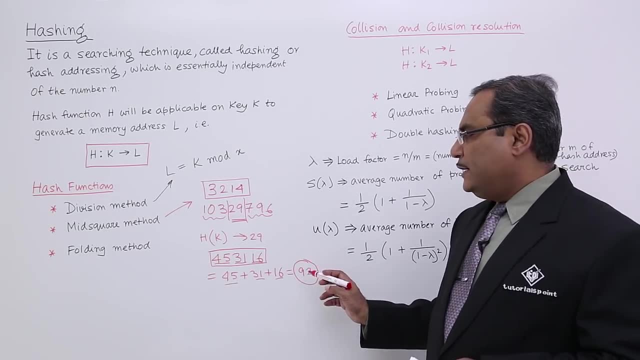 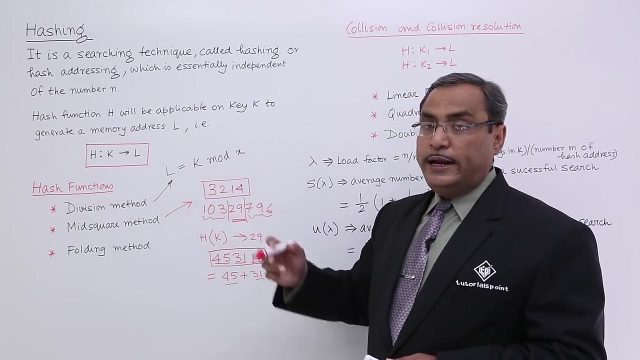 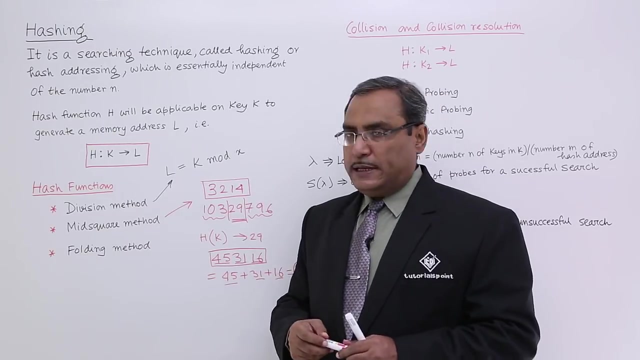 method. i'm just this number will be folded into three parts and then 453116 will get added. so now i'm getting this 92 and 92 is my l. so in this way we can apply this hash function on this particular k to get the required hash address or the value of l. so in this way this particular thing will take place. 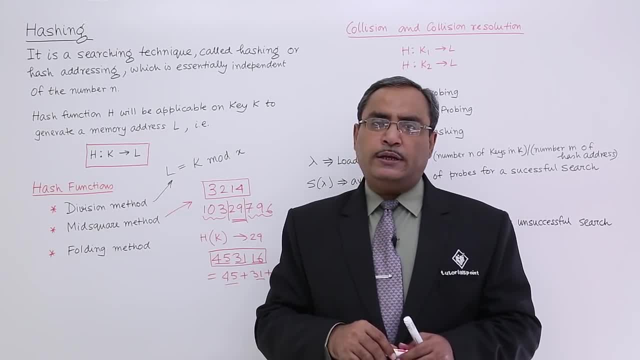 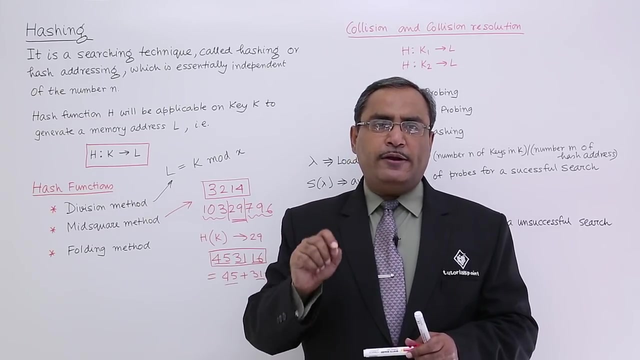 okay. now it is not mandatory that for different values for k, if we apply that hashing function it will generate different l. that may not be possible. so that means for different value of k, h of k can return the same l and that is known as the collision. and